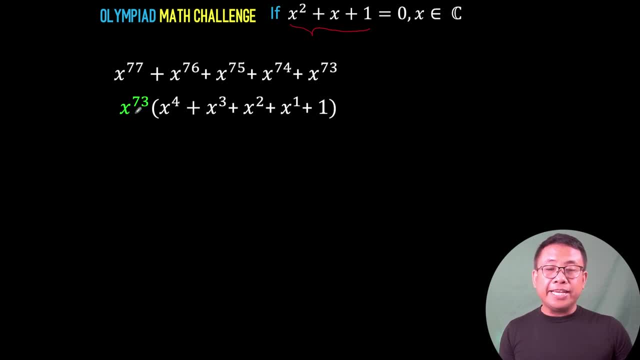 common factor is this result: The same explanation for each of those. Now look at this part. here You have x squared plus x plus 1, and compare that with this given equation: x squared plus x plus 1.. The result of this is equal to 0.. That means, instead of these: 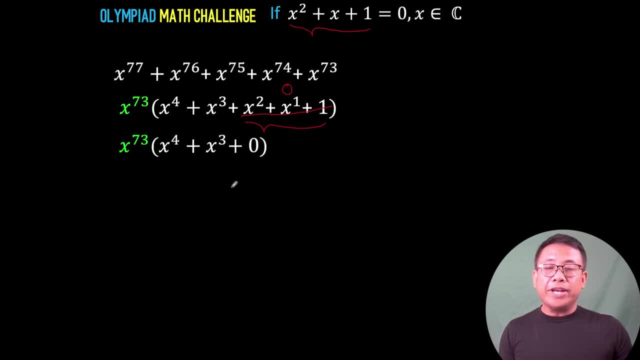 three terms. we can replace it with 0.. So what we now have is x to the fourth plus x cubed plus 0 for the second factor, and we just copy the first factor And of course you add 0 to any number. 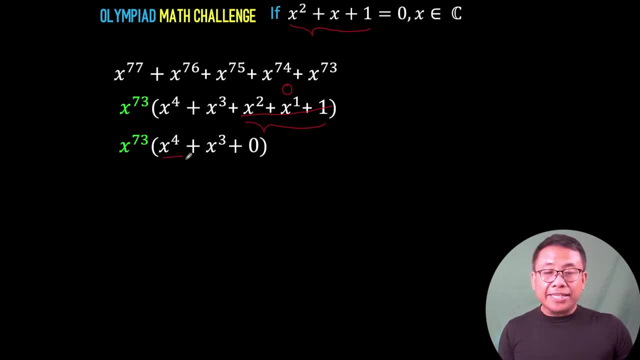 the result is still the same number. Now look at x to the fourth and x to the third. There is a common factor again of x to the third, which we factored out, and divide each of these terms by x to the third, We arrive at x plus 1.. This 0 is no longer written. Then we can multiply x to the 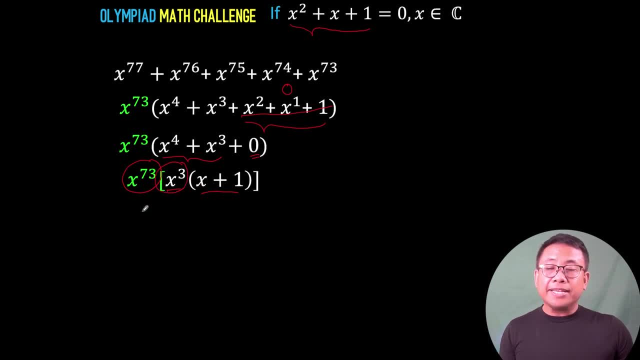 73rd plus x to the third, to arrive at x to the 76th, and we copy x plus 1.. Now we would like to know what expression can we use to get x to the third? So let's do that, Let's do that, Let's. 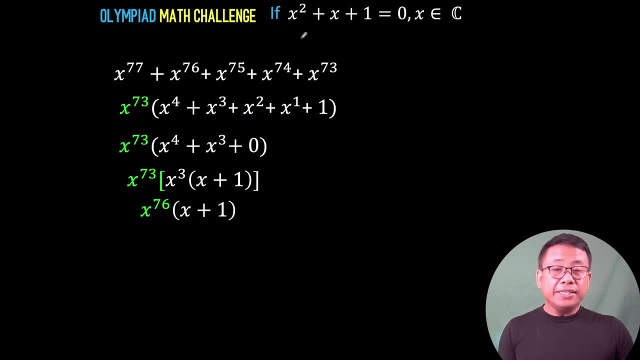 substitute for x plus 1 from the given equation here. So notice that x squared plus x plus 1 is equal to 0.. We now have this expression, x plus 1, similar to this x plus 1.. All we have to do is: 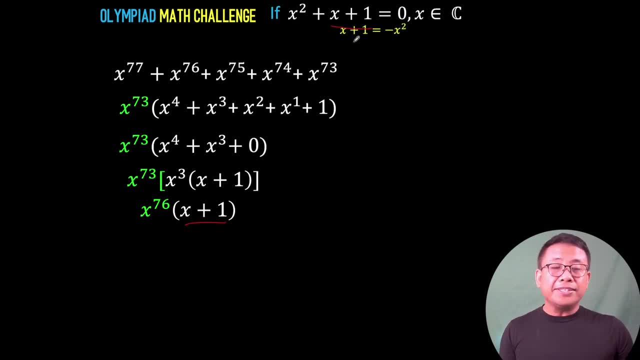 subtract x squared from both sides of the equation, And so we have: x plus 1 equals negative x squared. We can now replace this part by negative x squared, to have x raised to 76 times negative x squared in place of x plus 1.. And you have here a common base. 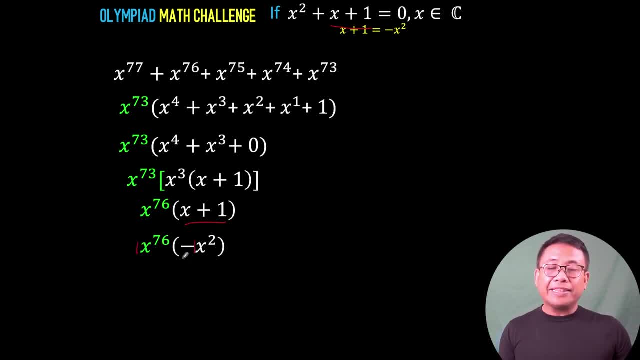 We're having a positive 1 here and a negative 1 here, So positive 1 times negative 1 is negative 1. And we copy the common base and we add the exponents 76 plus 2 to get 78. This is now. 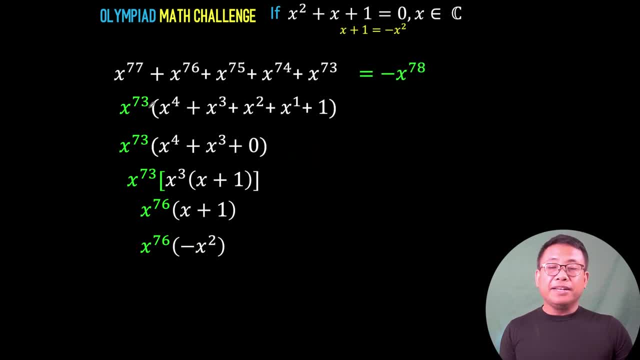 the value of this expression so far. Let's remove these other parts. This is not yet our answer, because we want to find the exact value of this given expression. Now let's recall the identity for the difference of two cubes. Now here, if we let a 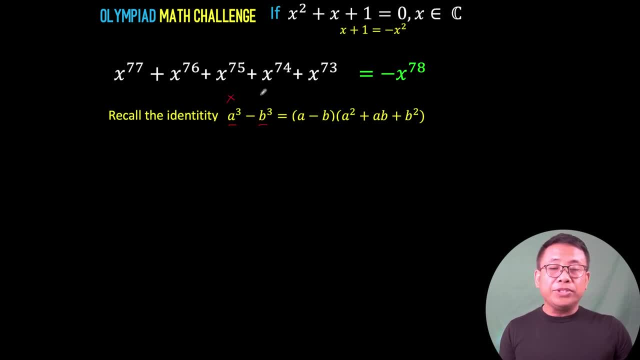 b equal to x and b be equal to 1, then if we take the difference of these two cubes, that would be equal to the first minus the second, that is, x minus 1 times the square of the first, which is x, squared plus the product of the first, and the second, which is x plus the square of 1 to arrive. 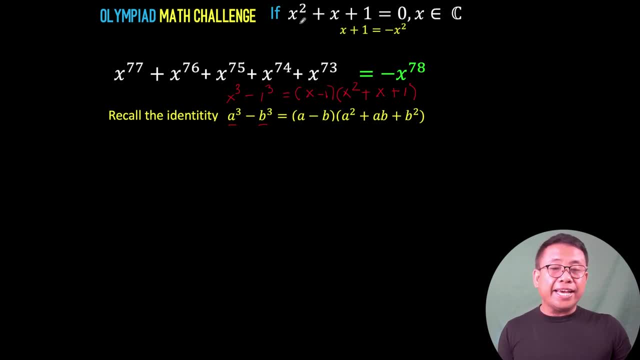 at this And notice that this x squared plus x plus 1 is again this given expression. So let's write it clearly, Let's remember that this 1 is equal to this and the value of that is equal to 0.. So again, we can. 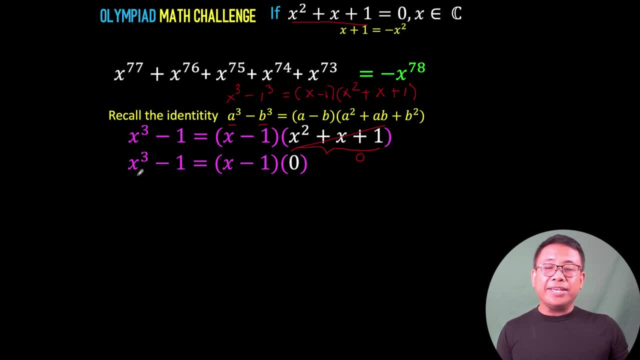 replace this with 0 and what's left with us now is x cubed minus 1 equals the quantity x minus 1 times 0. And since any number times 0 is 0, the right side is again 0. And solving for x cubed. 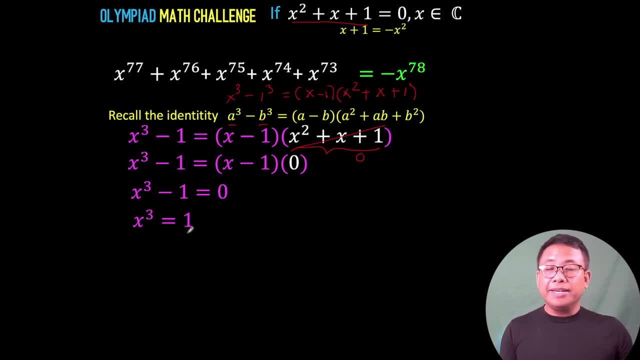 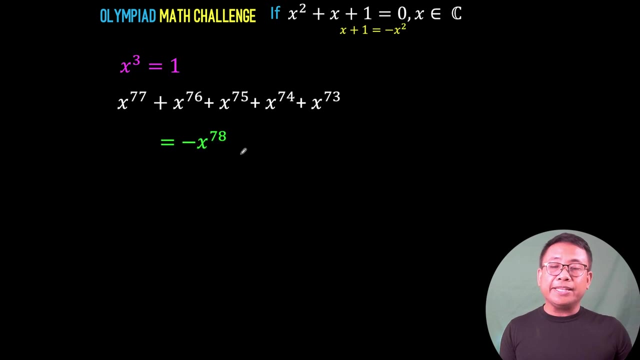 we add 1 to both sides of the equation to get x cubed is equal to 1.. So at this point we now know that x cubed is equal to 1.. So let's remember that value. Now, going back to this expression, negative x raised to 78, which is the value of the expression. 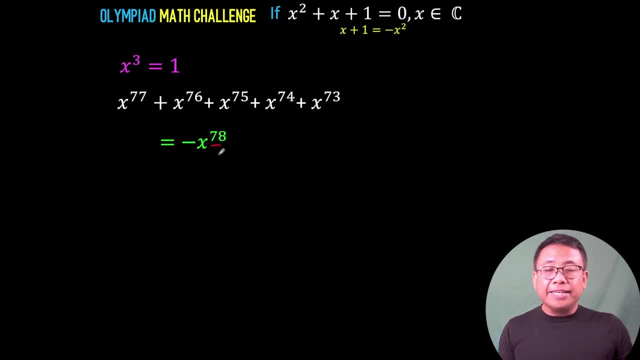 that we would like to find the value of Notice that this 78 can be written as multiples of this exponent 3, that is equal to 3 times 26.. In applying the power of power rule of exponent, then we can write this negative x raised to 78 as negative of x cubed raised to 26.. But what is the 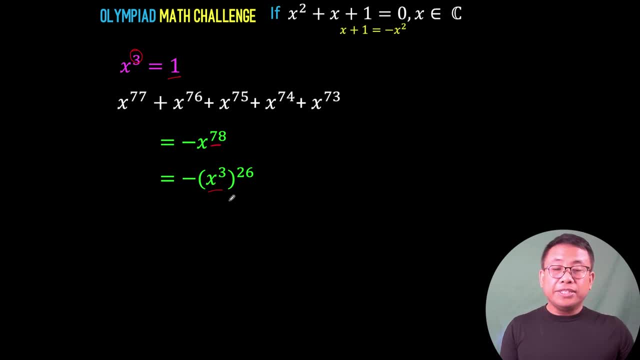 value of x cubed. x cubed is equal to 1.. So we can substitute 1 for x cubed to arrive at this, but 1 raised to 26 is still 1.. So, therefore, the value of this is simply negative: 1.. And that is now the value of the. 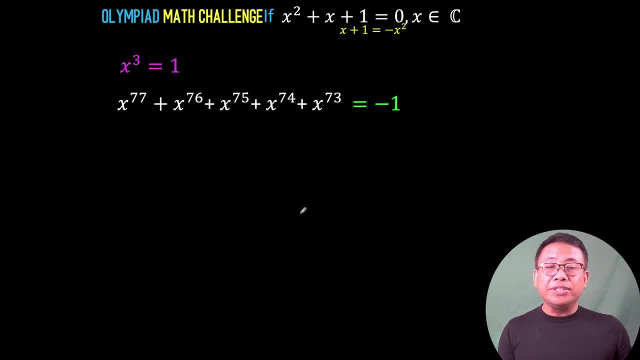 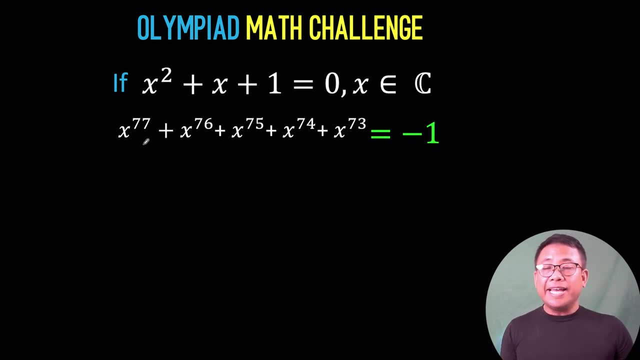 expression that we would like to find out. So going back now to our math challenge, if x squared plus x plus 1 equals 0 and x is an element of the set of complex numbers, then x to the 77th plus x to the 76th plus x to the 75th is equal to 1.. So we can substitute 1 for x cubed to arrive at this. 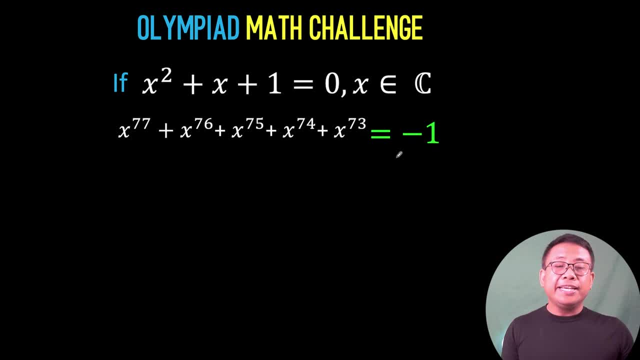 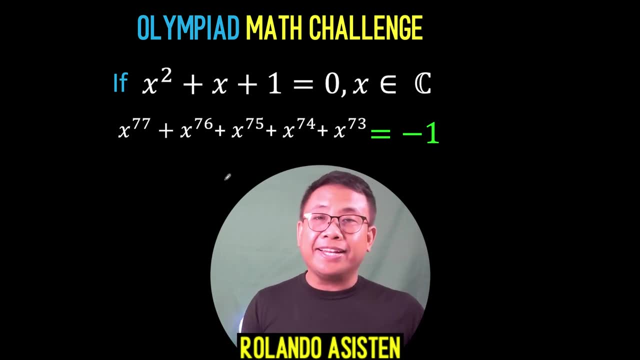 plus x to the 74th, plus x to the 73rd is now equal to negative 1.. And this problem is now solved. So thank you very much. This is Lando Assistant and we hope to see you again in our next video. Bye for now.